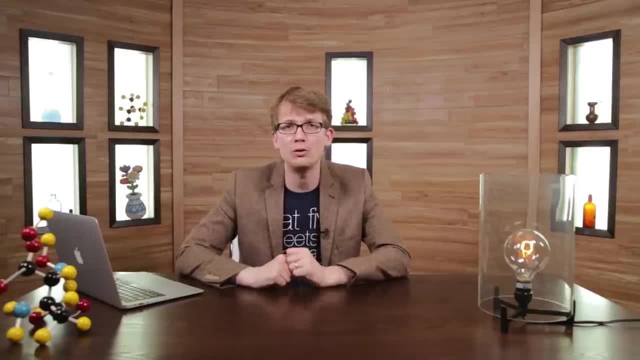 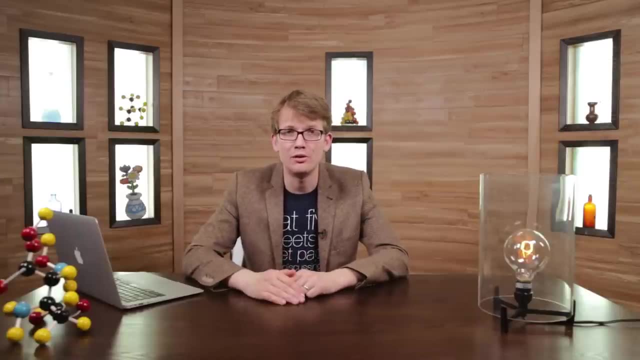 The branch of chemistry that studies how these collisions affect the rate of reactions is kinetics, and, if you ask me, it's just as exciting and a heck of a lot more useful than demolition derbies. If only they sold funnel cakes in chemistry class. 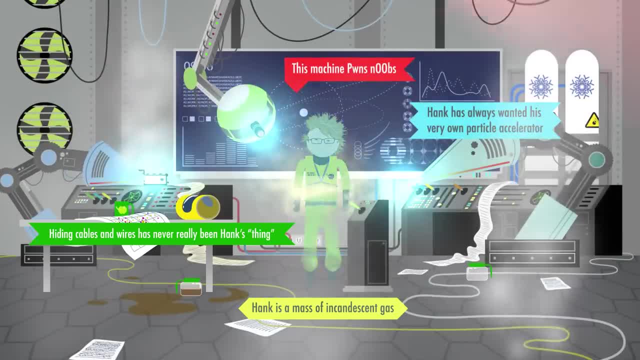 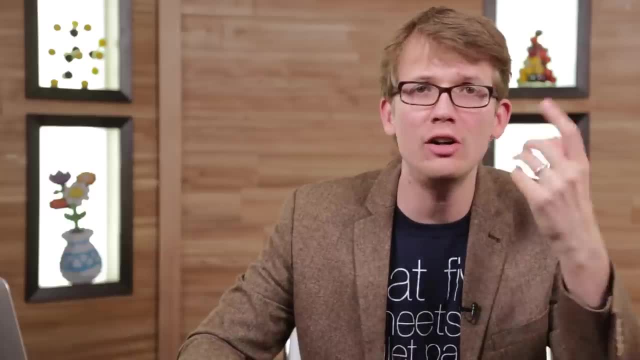 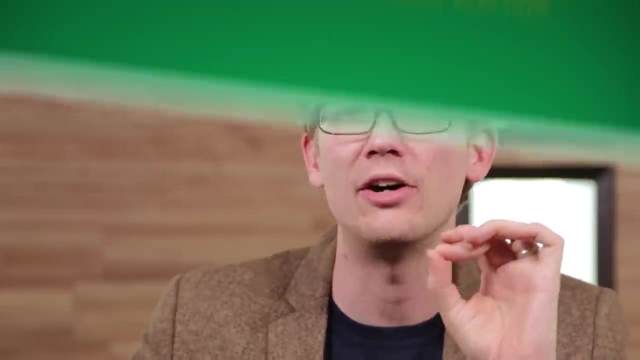 So if chemical reactions only work when particles bang into each other good and hard, just how hard do they have to bang into each other? Every reaction has a minimum amount of energy required to get it started. This is known as the activation energy. 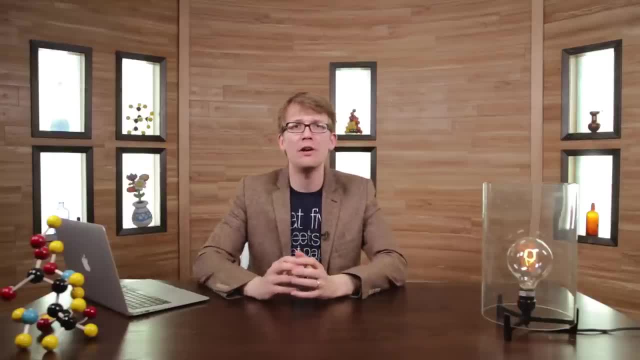 Molecules require this much energy to hit other molecules hard enough to break them apart and reform them in different ways. Without it, nothing will happen. It's like a hill that you can climb up to. It's like a hill that you can climb up to. 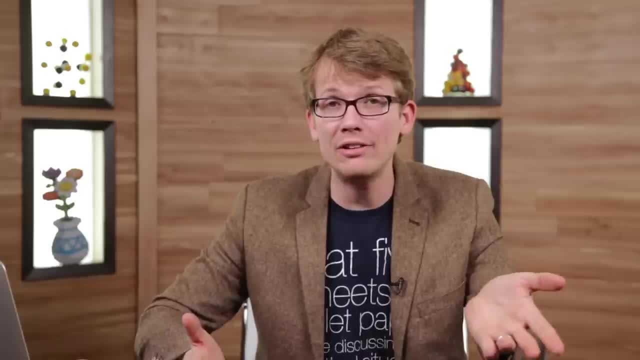 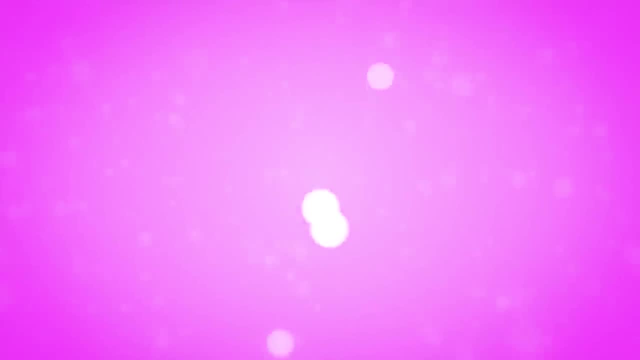 It's like a hill that you can climb up to that molecules have to get over before they can go any further. So where do they get this energy? Well, it's kinetic energy, the actual speed of the particles. So just like the cars at a demolition derby, all else being equal, the faster the particles. 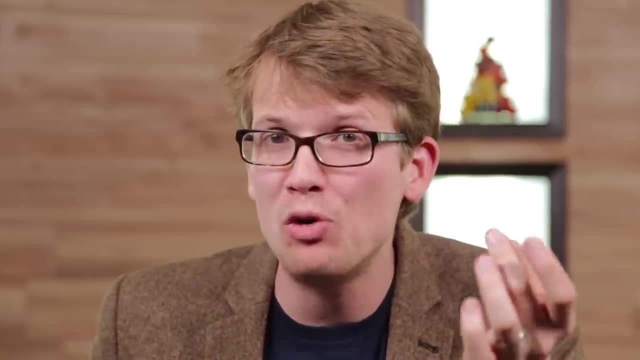 move, the harder the collision will be. But still, no matter how hard they hit, it won't do any good if they're not hitting the right way in the right places. Like if you keep smashing into the back of a guy's trunk, that's not going to stop. 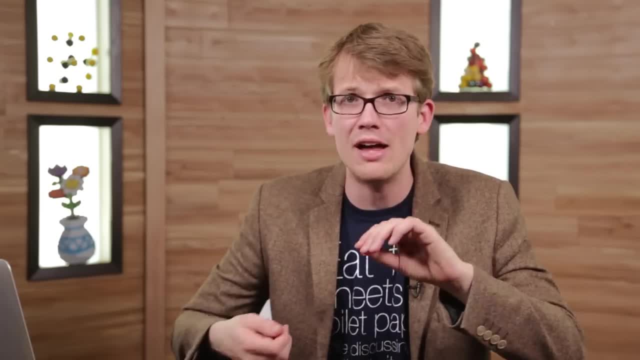 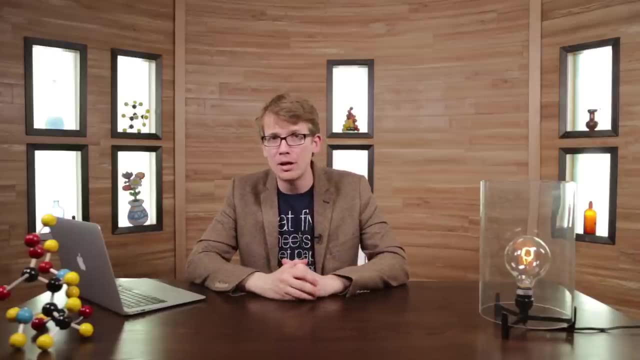 his car. There's no engine back there. You can bang Velcro together all day and night, and if it's not turned the right way, it'll never stick together. Same thing with molecules As an example. take nitric oxide, one of the byproducts of gasoline combustion, and something 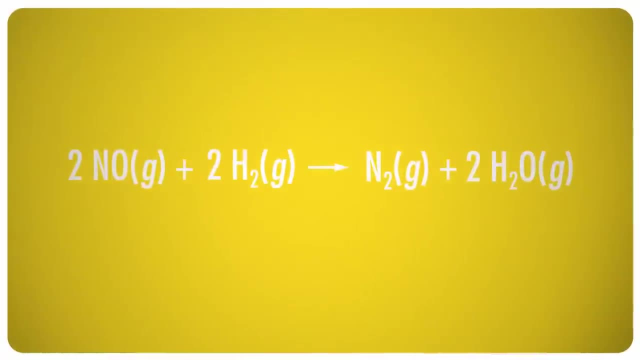 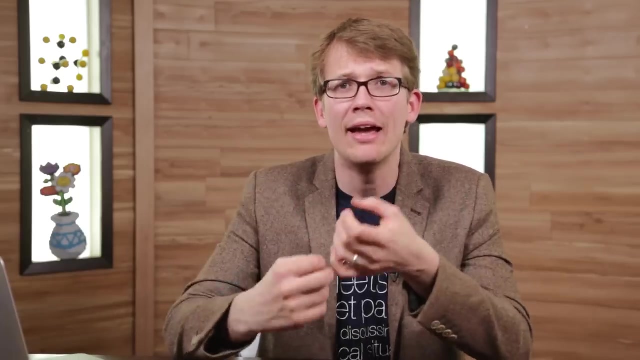 that you can smell quite clearly at a demolition derby. Under the right conditions it reacts with hydrogen gas to produce nitrogen gas and water. But the molecules have to hit each other- just the right way To make N2,. two NOs have to collide in such a way that the nitrogens are together. 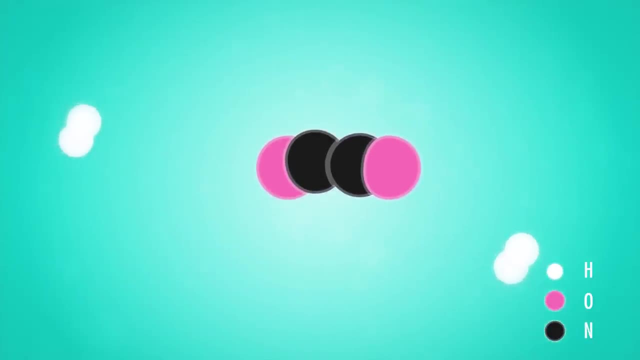 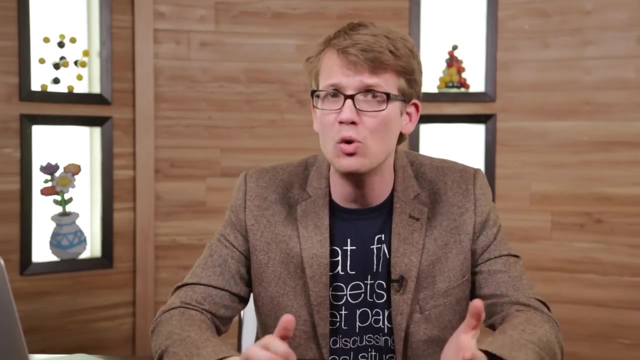 And to get H2O, a molecule of H2 has to collide with the oxygen side of an NO molecule, Just like Velcro being turned the wrong way. You can smack the H2O in the same way. You can look at the inside against the H2 all day and you'll never get any water from. 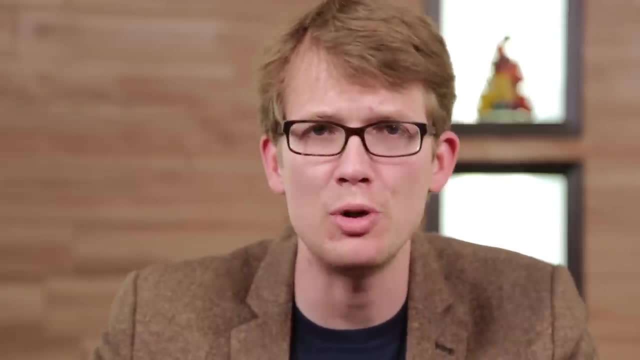 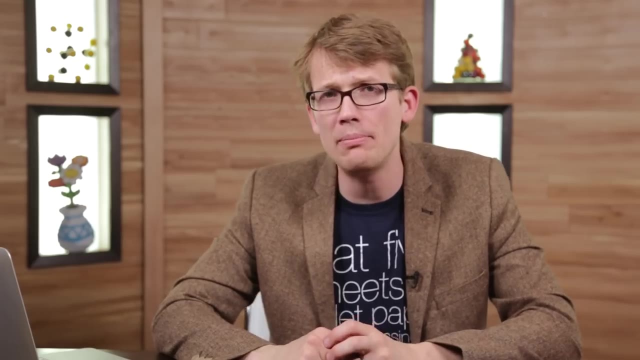 it. Now. let's say that we're having a lot of solid effective collisions between the molecules. The reaction should hum along with no further hindrances, right? Well, yes and no. Once the energy requirements are met, the reaction will proceed. 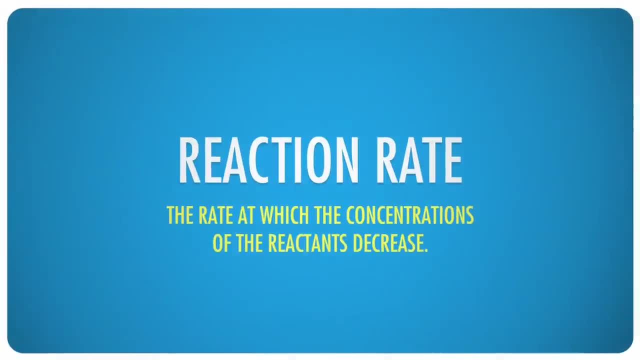 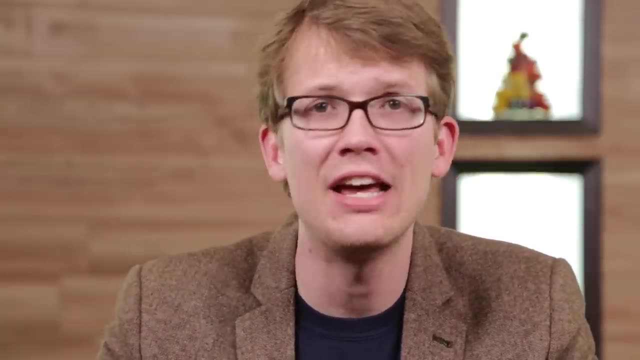 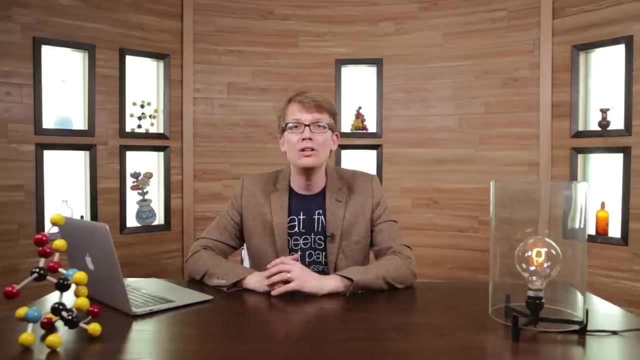 But its speed or reaction rate will vary wildly from super-fast to super-slow. So the reaction rate, that's the rate at which the concentrations of the reactants decrease- And this has to be determined experimentally- can't be calculated from the energy change or any other thermodynamic factor. 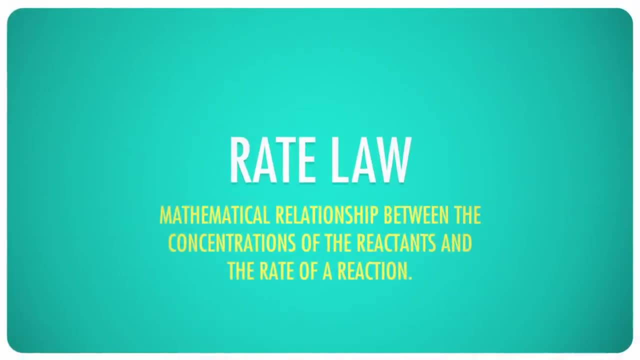 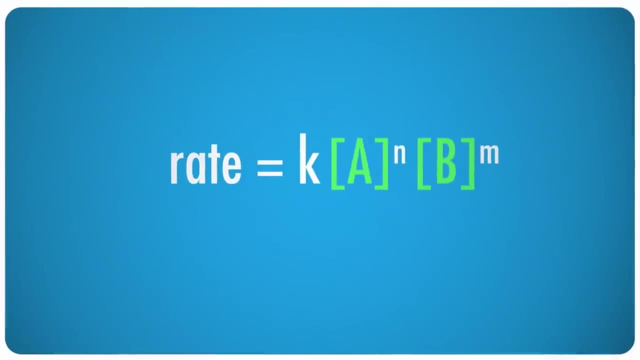 One useful way to think about the rate is a quantity called the reaction's rate law. It describes the relationship between the initial concentrations of the reactants and the rate at which they react. The rate law for a reaction is written like this: The rate equals a constant K times the concentrations of each reactant raised to some power. 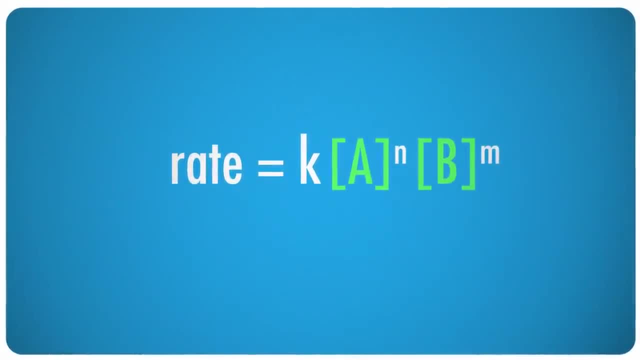 Notice that only the reactants are used for this, not the products. The rate law for a nitric oxide reaction then ends up as K times the nitric oxide concentration raised to some power, times the hydrogen concentration, also raised to some power. So you're probably wondering about all those raised to some power. 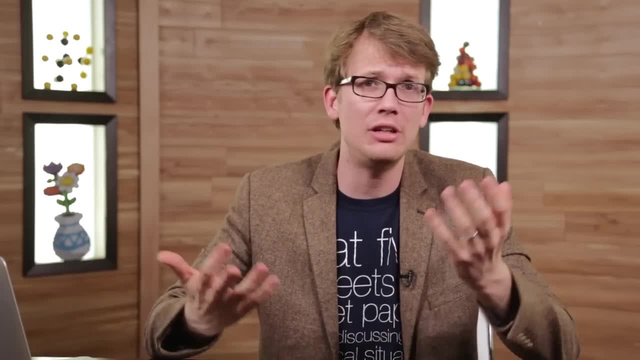 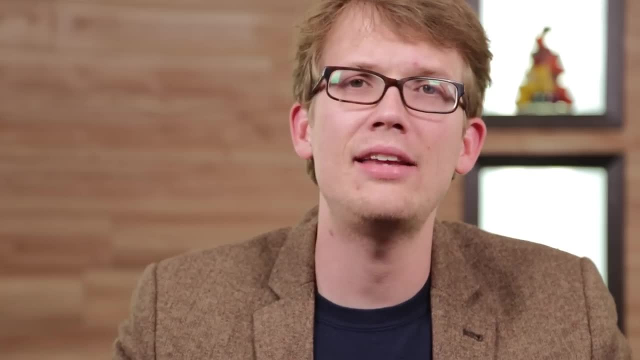 Like what power? And you should be wondering that The exponents in rate laws are tricky even for professional chemists and engineers because, like I said, they can only be determined experimentally. It's kind of intense, but we can handle it. 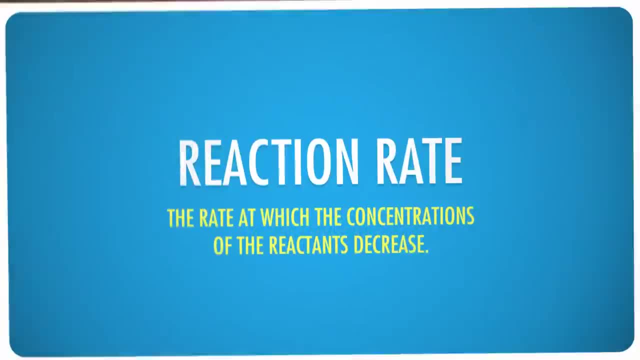 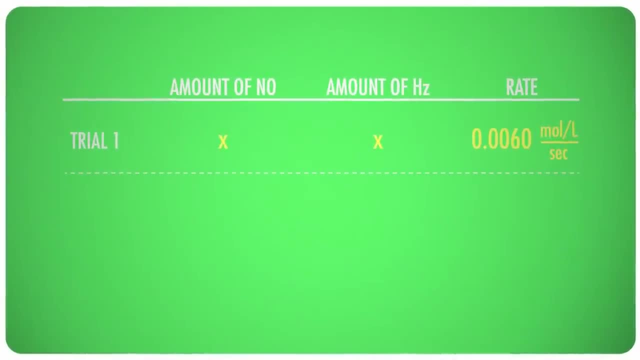 Check it out. Suppose we did the reaction a few different ways and calculated the rate for each instance. Let's say That with the first reaction we got a rate of 0.0060 moles per liter per second. Then we repeat the reaction with the same amount of nitric oxide, but this time with 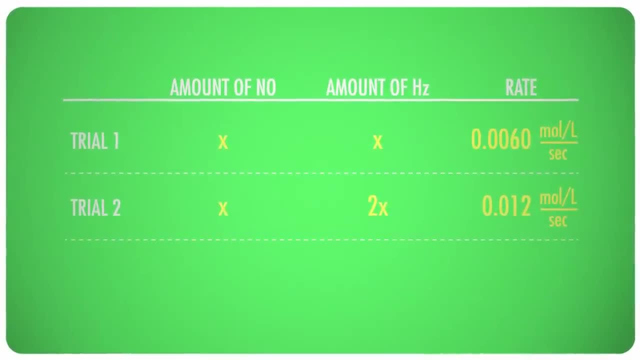 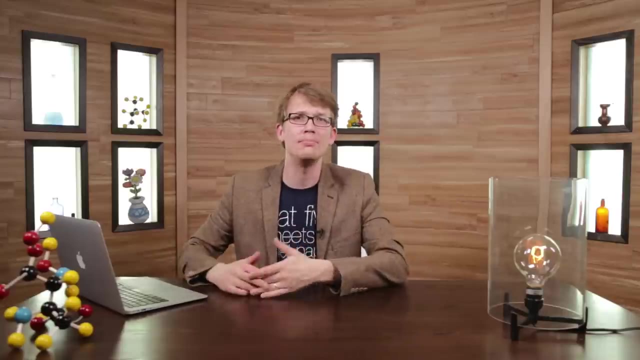 twice as much hydrogen as before, And now we find that the rate of the reaction is 0.012 moles per liter per second. What does this tell us? Well, doubling the hydrogen, doubled the rate, meaning that the rate and the H2 concentration. 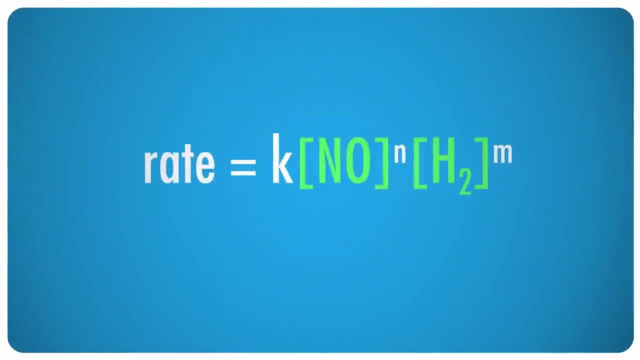 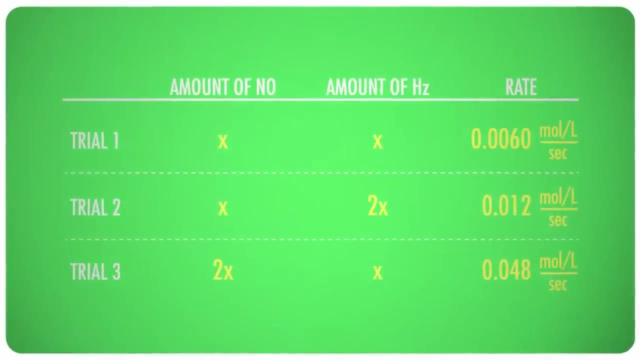 change in exactly the same way. So in the rate law, this can be expressed by the concentration being raised to the power of one. Finally, we do it one last time. with the original amount of hydrogen, We get twice as much. NO, and this time we find that we get a rate of 0.048 moles per. 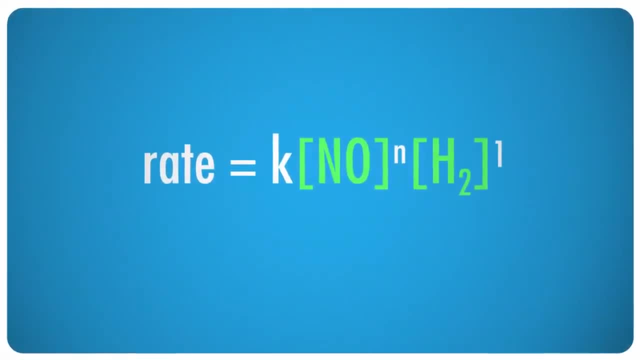 liter per second. Doubling the nitric oxide caused the rate to increase by eight times, and that can be expressed in mathematical terms by cubing the concentration term. This means that the final rate law for this reaction is K times the concentration of hydrogen. 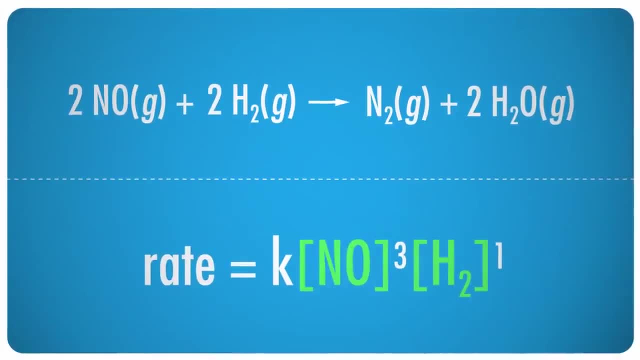 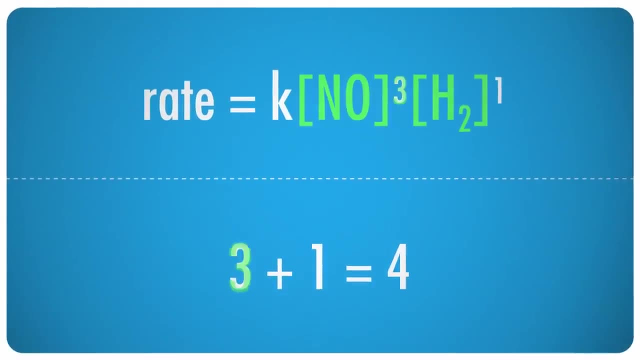 gas to the first power. you don't need to write out the one obviously times the concentration of nitric oxide cubed. A rate law in this form is said to be of the fourth order. We get that value by adding the exponents together: three plus one. 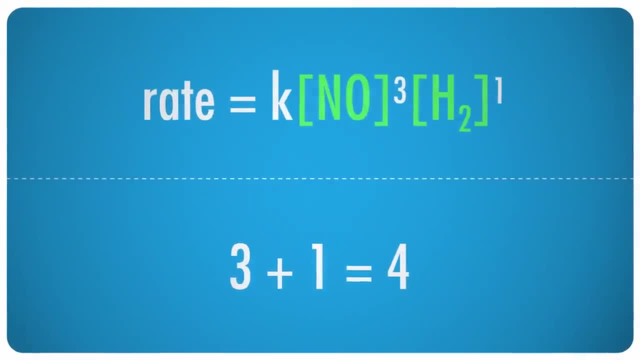 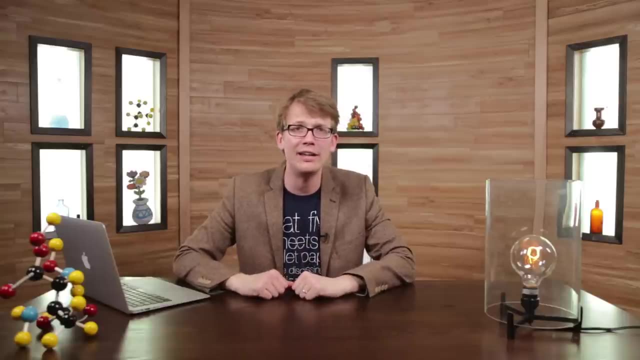 There is some math that isn't hard here. That equals four. Fourth order reactions are actually quite rare. Most reactions are of the zero, first or second order, but in all cases it's calculated exactly as we have done here. Now, if you've watched our episode on equilibrium, this formula should look familiar to you. 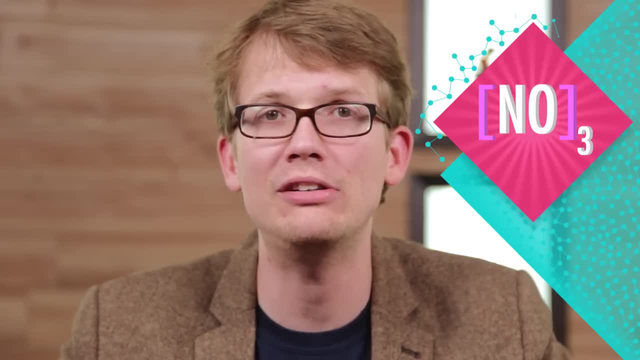 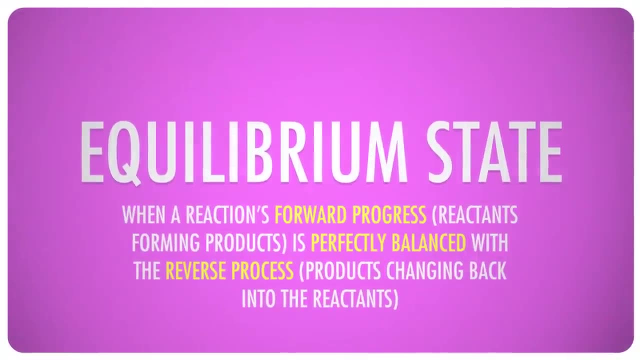 Equilibrium expressions also use bracketed concentrations with exponents, and that's no accident. Those formulas come from these ones. A reaction is at equilibrium when its forward and reverse rates are equal right. Well, if we were to find the reverse rate law for a reaction, it would take the same. 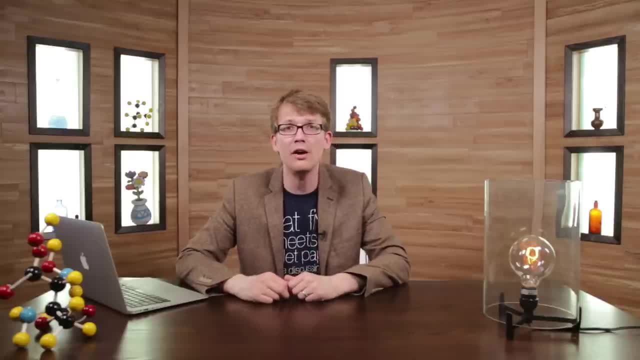 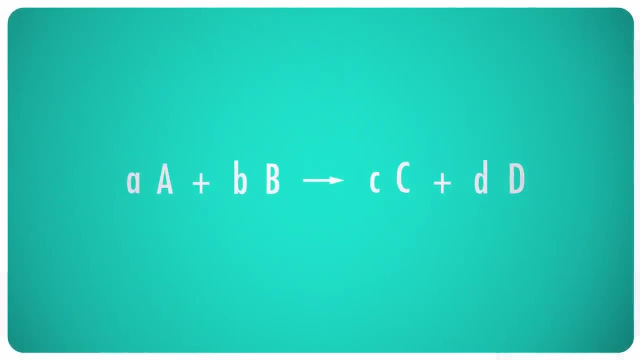 form as the forward one, but using the initial concentrations for the products rather than the reactants. Think of like an imaginary reaction: A plus B yields C plus D. The lowercase letters represent the coefficients of the reactants and products. The forward rate law is K times the initial concentration of A raised to some power times. 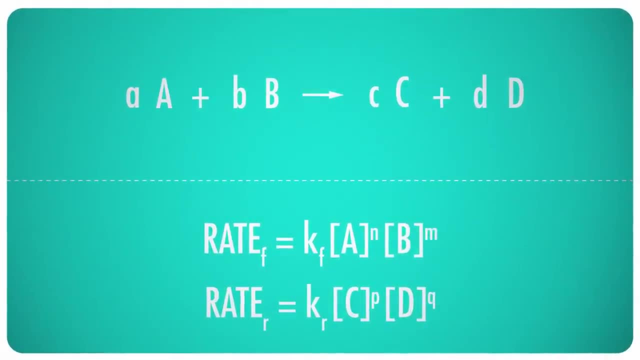 the initial concentration of B raised to some power, And the reverse is the same, but with C and D in place of A and B. Notice that these exponents are not, however, the coefficients of the balanced equation. If we write these two terms together to show that the forward and reverse rates are equal, 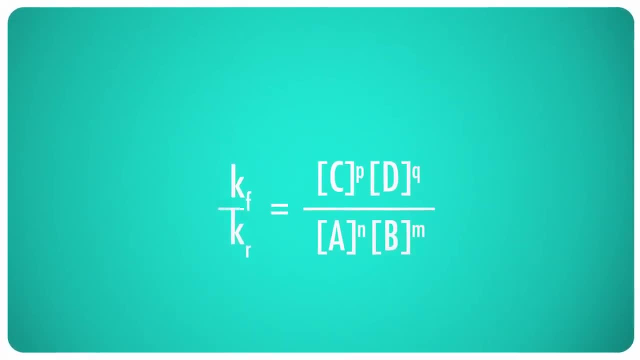 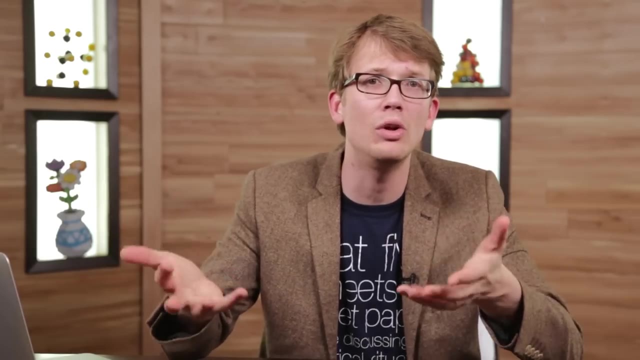 like at equilibrium and solve for a single constant, we get something that looks very much like an equilibrium expression. For mathematical reasons, the exponents don't translate. but yeah, basically this is where the equilibrium equations come from. Pretty cool, But if it's that simple, why don't all reactions just go to an equilibrium state? 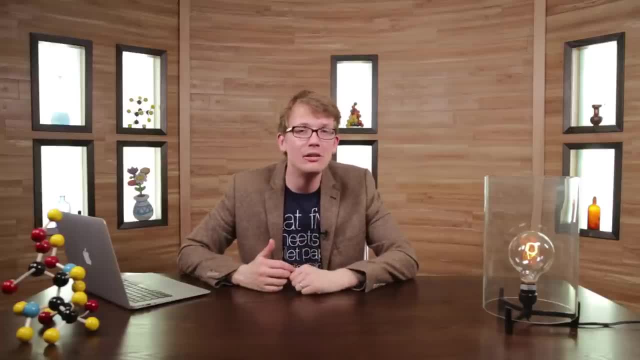 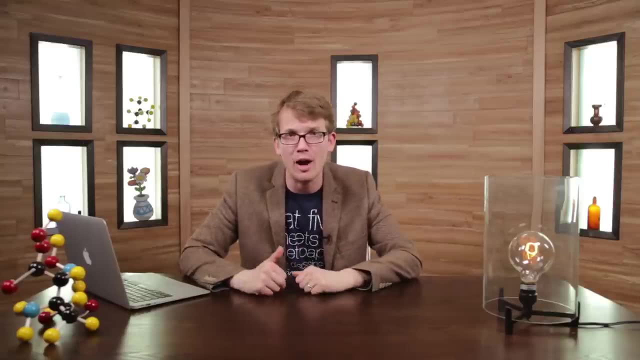 and stay there. Well, sometimes the reverse reaction isn't thermodynamically spontaneous for one reason or another. Sometimes the forward reaction is so vigorous that any reactants that might reform are immediately pushed back into products, Or the products might physically separate and have little chance of colliding at all. like when products separate into solids and gases. Often, though, it's just that the reverse reaction has such a high activation energy that the collisions are almost always ineffective, Because- remember- most reactions don't happen instantly boom all at once. Instead, they happen in steps. 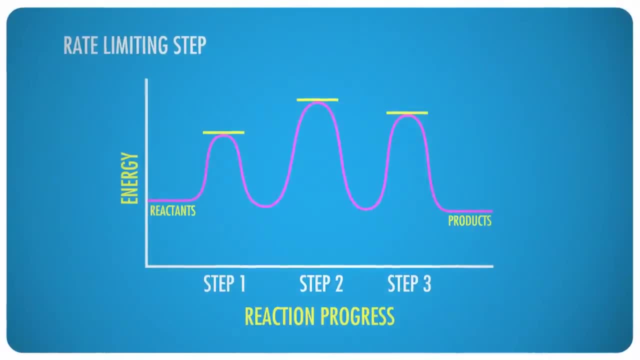 And, as with any multi-step process, the reaction can only happen as fast as it takes, And that's what we're going to talk about in this video. The slowest step is the one that has the highest activation energy, And sometimes that step is very slow indeed. 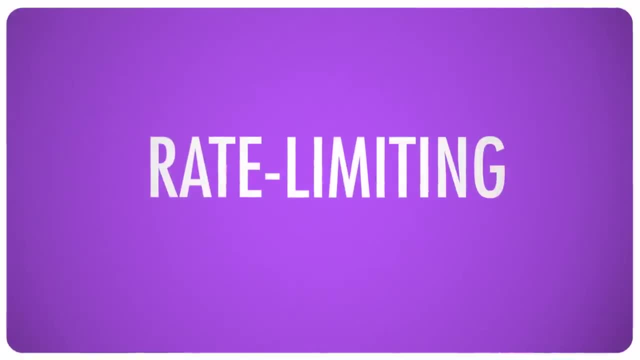 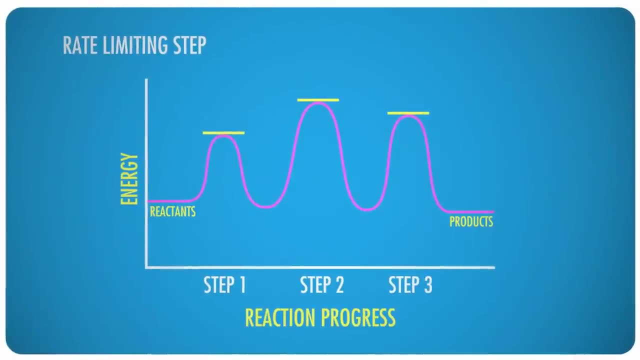 Since it's what controls how fast everything else can go, we call it the rate-limiting or rate-determining step. The slowest step is the one that has the highest activation energy. If the particles have trouble getting over that part of the energy hill, then they'll. 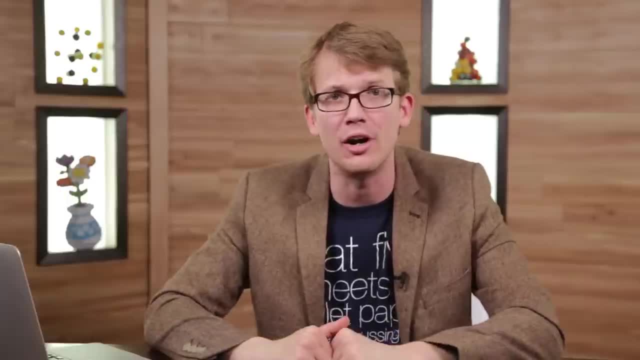 have trouble making it to the finish line, no matter how fast the other steps are. So in the case of the nitric oxide reaction we've been discussing, there are actually three steps. First, the nitric oxide and the H2 form water. 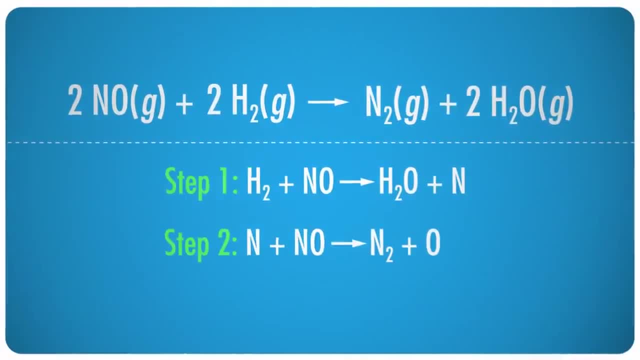 Then the nitrogen combines with another molecule of NO to form N2 and elemental oxygen. Finally, that atom of oxygen combines with another molecule of H2 to form water. Here step two is the slow one, And no matter how fast you take the first step, the water product can never be produced. 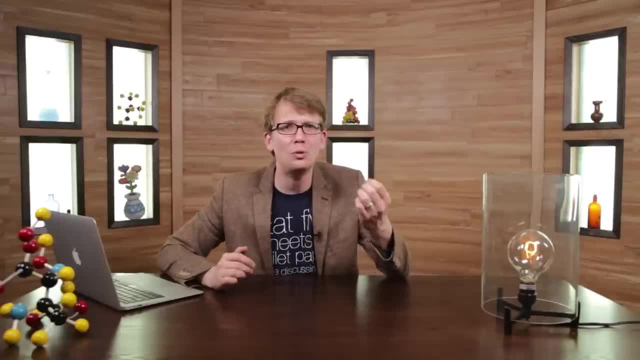 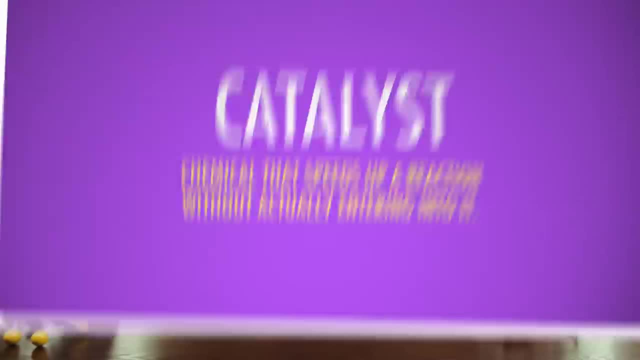 until the nitrogen gases. The problem is, we can't always afford to wait around for reactions to happen on their own. Sometimes they need to be forced along, And that's the job of catalysts. A catalyst is a chemical that lowers the activation energy of a reaction, thereby speeding it. 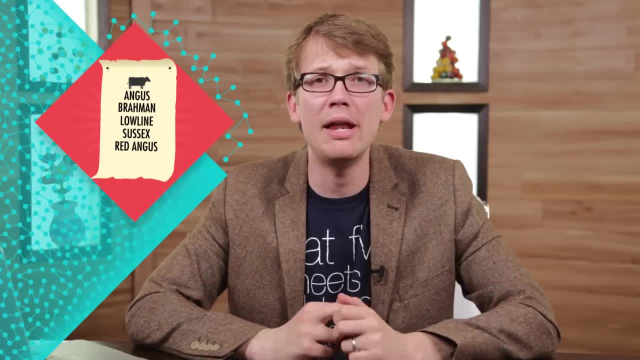 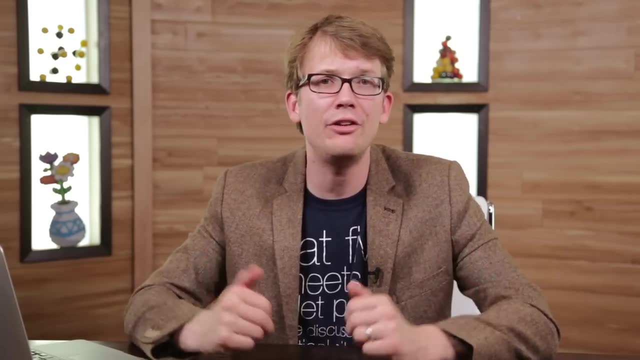 up without actually being changed by it. Catalysts take many different forms. They can be just another chemical added to the reaction vessel, a piece of metal that's in contact with the reacting chemicals, or even a gas that's added to the environment. 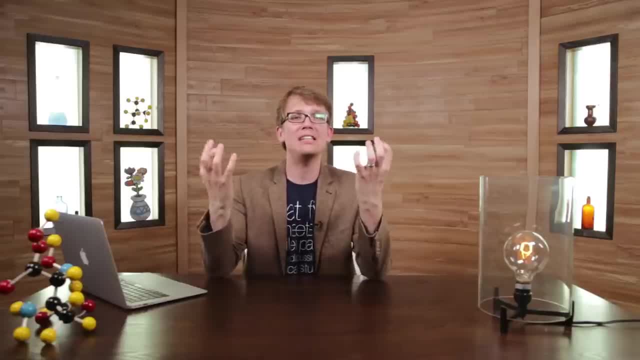 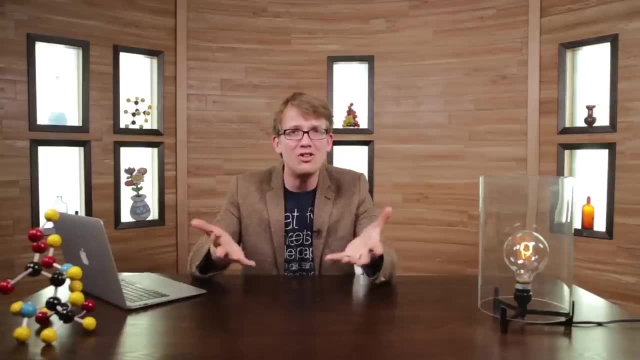 One of the most common and important classes of catalysts are the enzymes in living things. Without them, many of the chemical processes that our bodies must do every day to keep us alive would slow essentially to a stop. We literally have to stop. 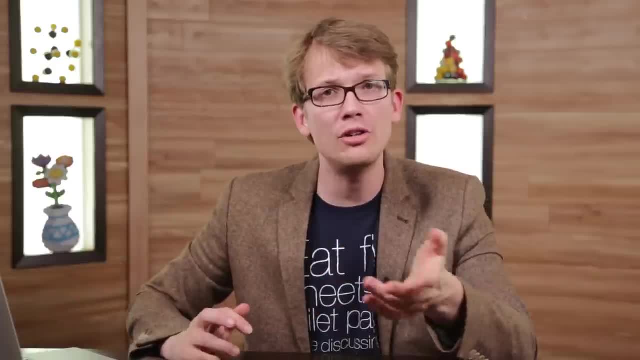 We have to stop. But we know that they could not survive without them. So there you go. In demolition, derbies and in chemistry, it all comes down to how hard you can hit and how well you can aim your punches. 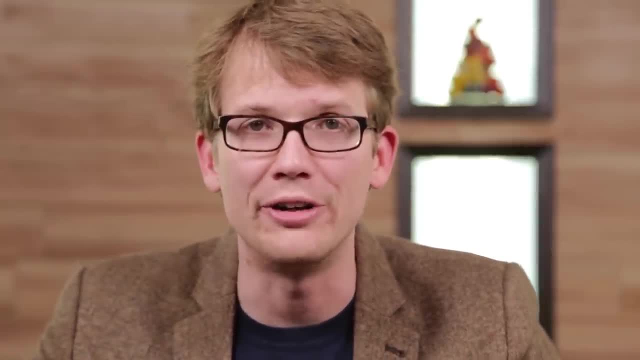 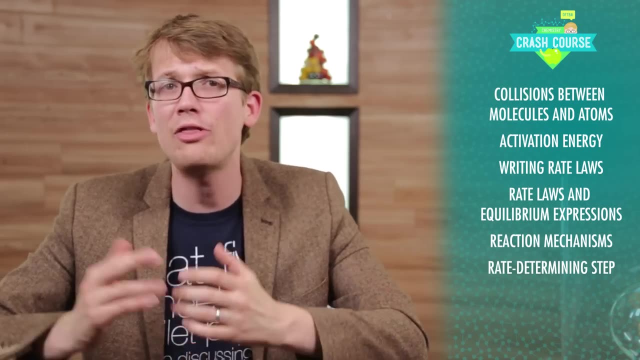 Chemistry Surprisingly exciting even without funnel cakes. Thanks for hanging out for this episode of Crash Course Chemistry. If you paid attention, you learned that chemical reactions depend on collisions between molecules and atoms, that the particles have to be oriented correctly when they collide and that they 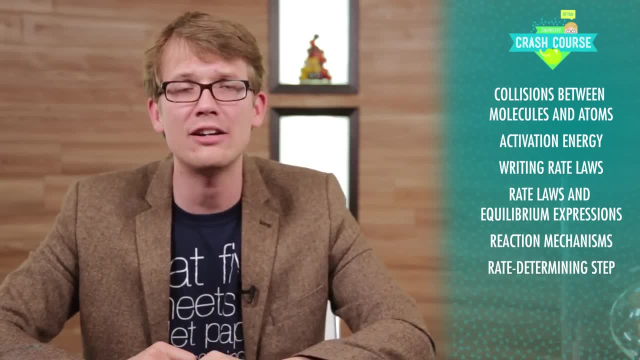 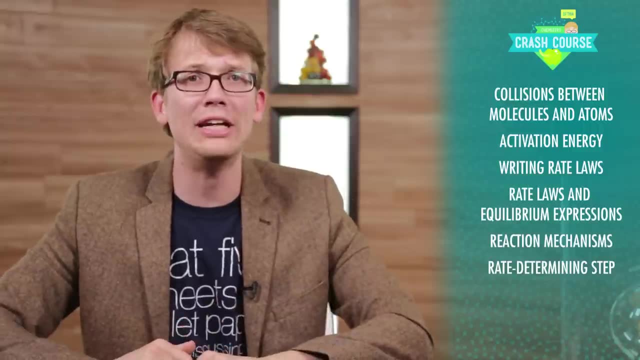 have to collide with enough energy to meet the threshold for the reaction known as the activation energy. You also learned how to write rate laws and figure out their initialward Modelwedder comes up from this exponents and how to calculate the form or order of a rate law. 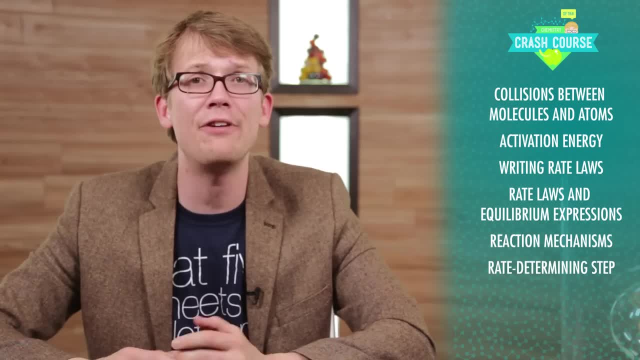 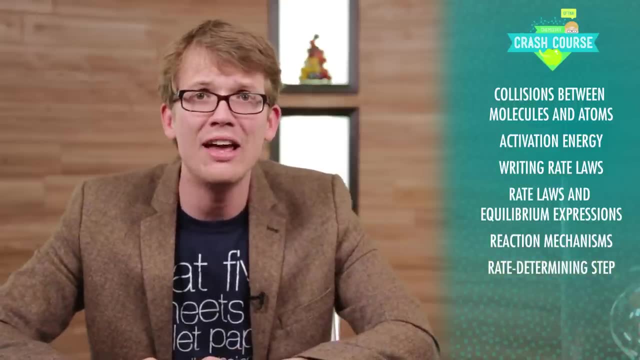 You learned how rate laws are related to equilibrium expressions. And finally, you learned that chemical reactions actually happen in steps, that the slowest step determines the overall rate of the reaction and that the reason for that comes right back around to the activation energy.